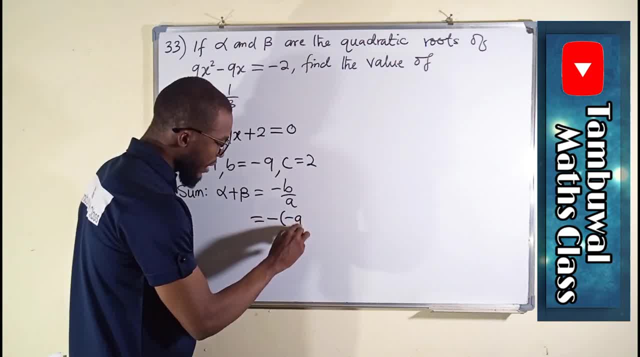 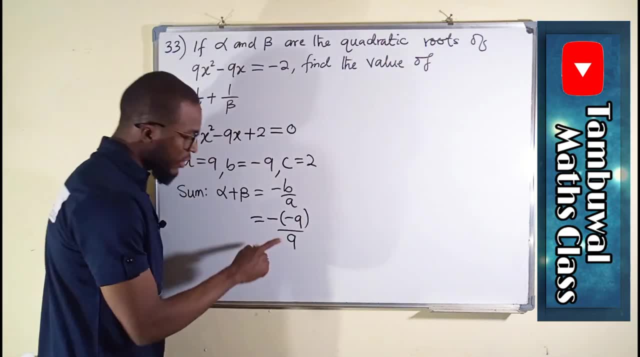 negative. So we have negative negative, 9 over a and a. here is what: 9.. Altogether, this negative will change this to positive, because negative negative is positive. 9 divided by 9 is 1.. So the sum is equal to 1.. 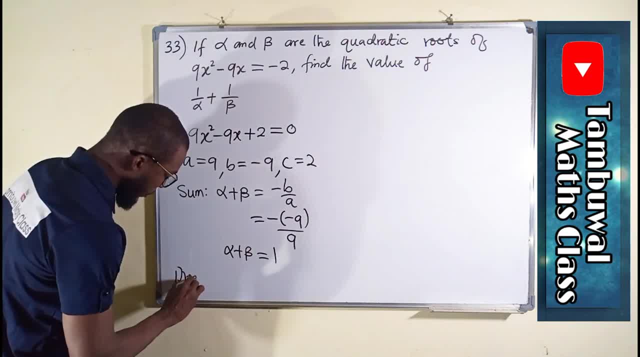 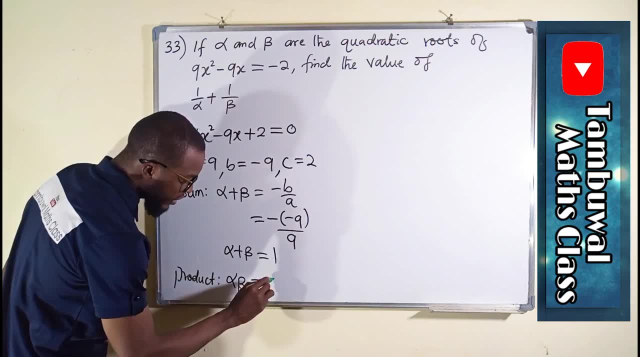 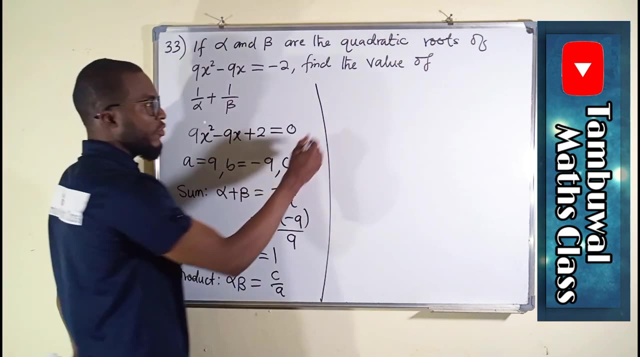 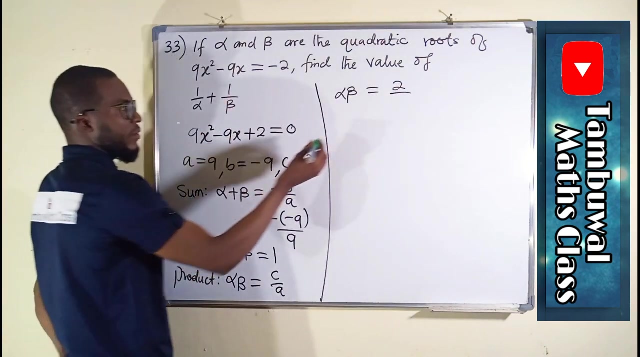 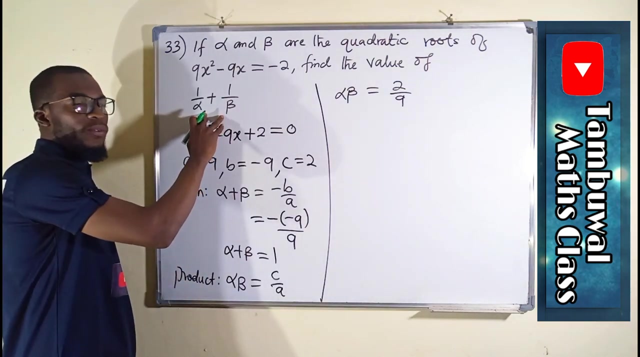 Therefore the product. we should multiply them together. Alpha times beta can be obtained by taking c over a, and our c is constant. you can see it here as 2, so alpha times beta will be equal to 2 over a. our a is 9. so, having obtained this, let us simplify this, because this is what we are looking for. 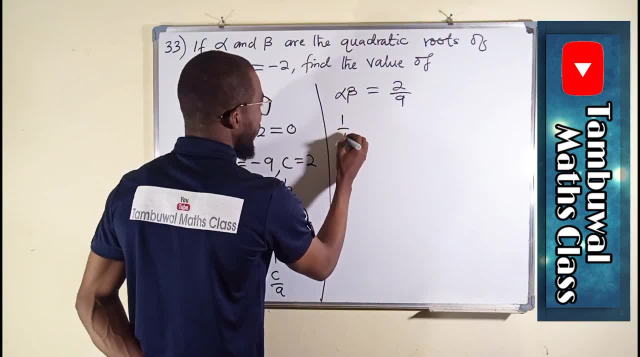 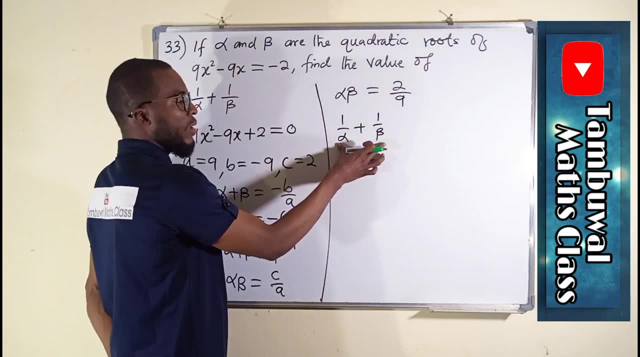 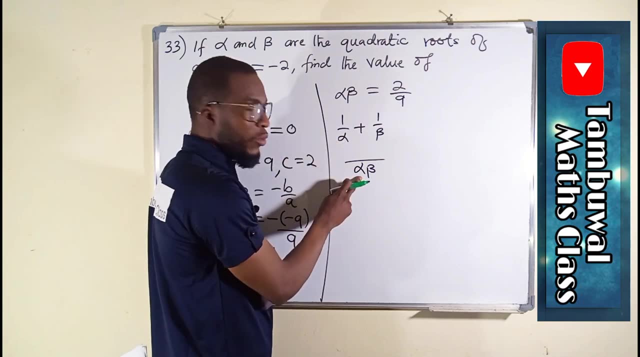 we are looking for 1 over alpha plus 1 over beta, the LCM between them. if you take the LCM of alpha and beta, you should obtain alpha beta. when you take alpha and plug it here, you're going to obtain beta and beta times 1 is beta. 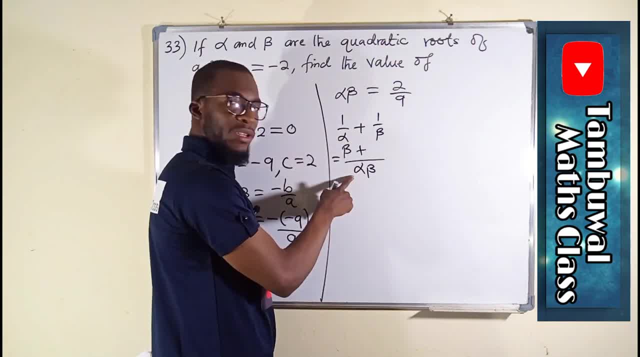 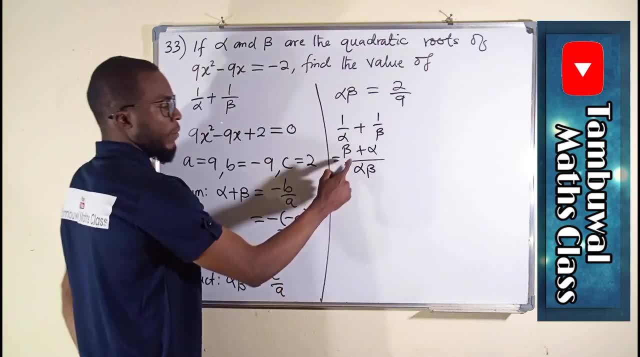 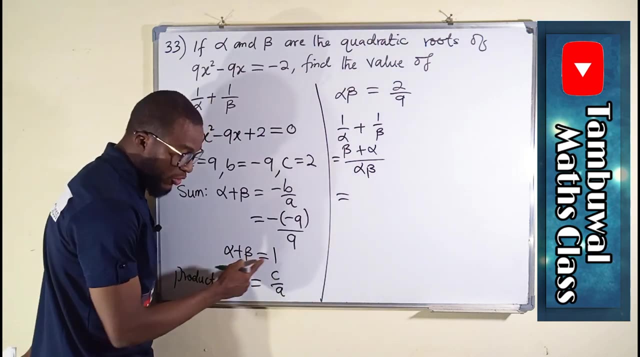 plus, when you take beta, plug it here, you're going to obtain alpha, and that alpha times 1 is alpha. this is equal to beta plus alpha is the symptom of saying alpha plus beta. they are commutative. we have alpha plus beta to be equal to 1 here, so we have 1 here. 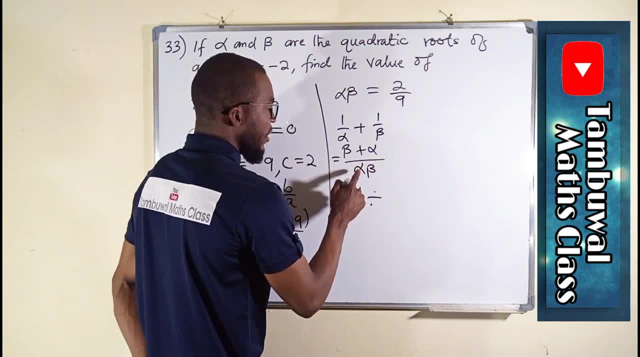 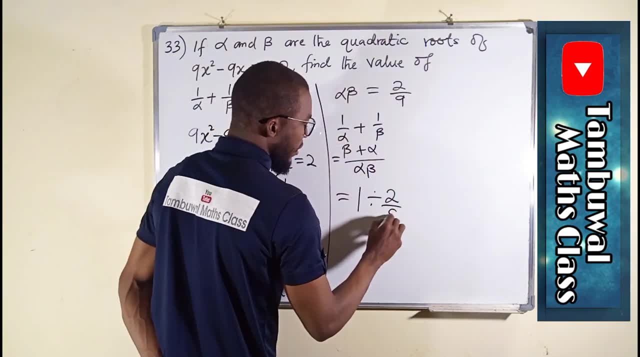 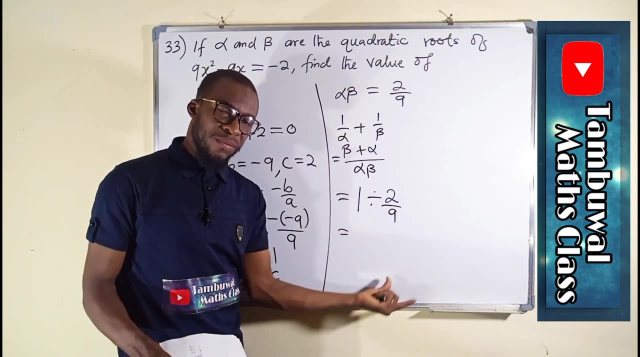 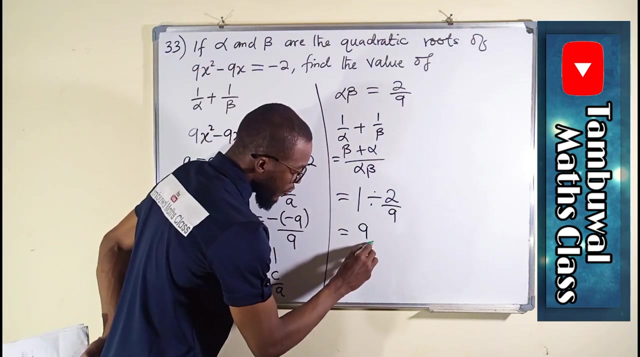 divided by. because this is a division sign, alpha times, beta, we have it here as 2 over 9, 2 over 9. this is equal to. this is a fraction, and 1 is divided by our fraction is just like taking the reciprocal of that fraction by flipping it over as nine over. 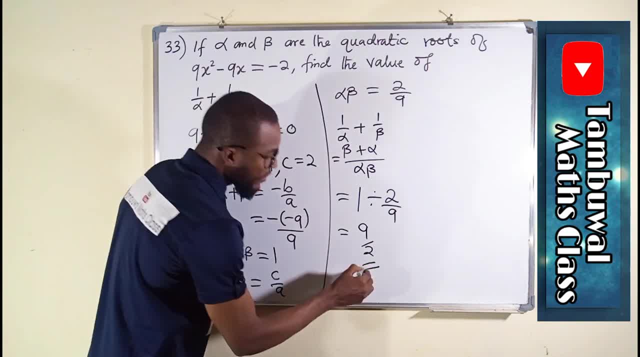 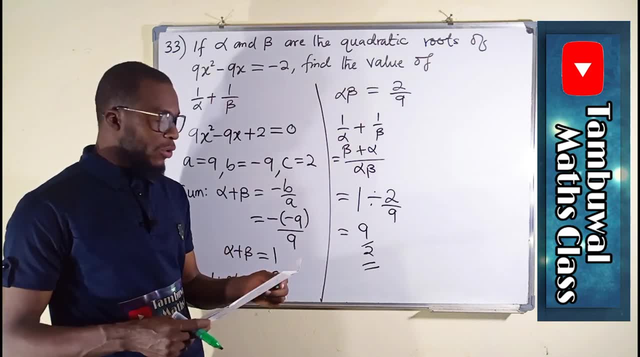 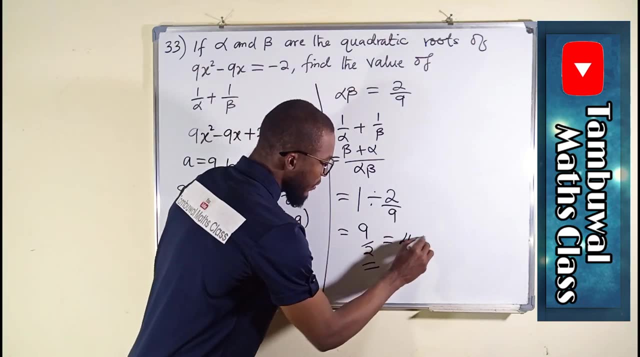 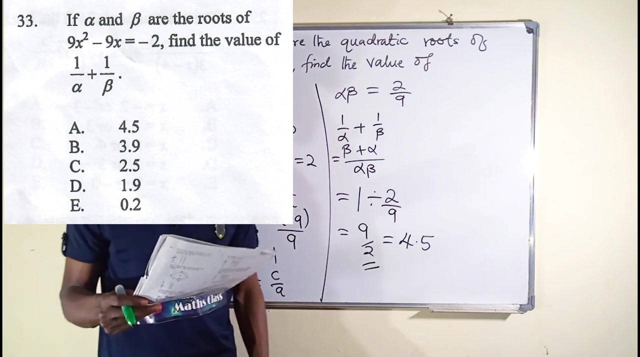 two instead of two over nine, and this is the required solution- nine over two- and improve our fraction. okay, all the solutions here are in decimal points, so let us see how we can change it. this one is the same thing as 4.5, which is option a here. so now let us look on to question number 34.